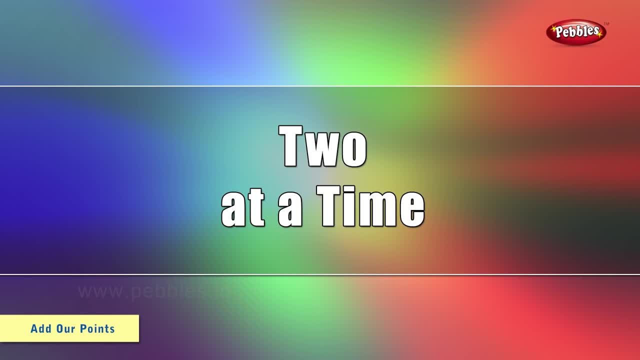 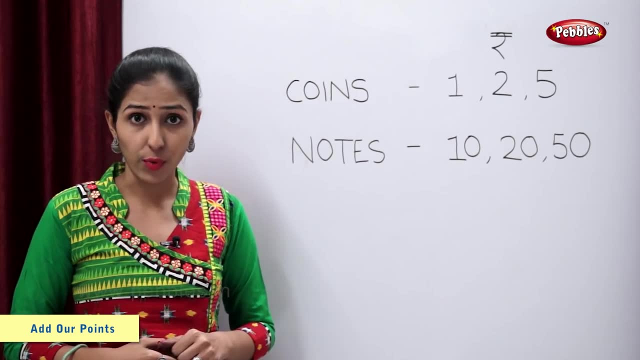 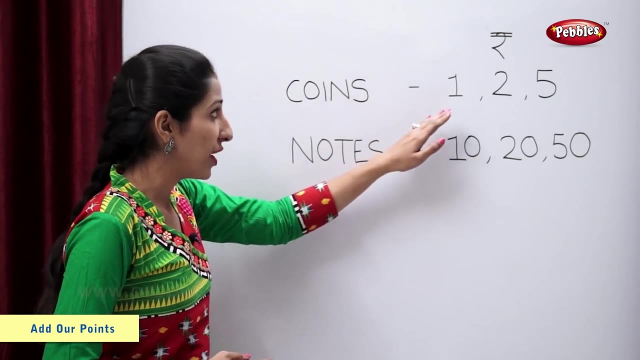 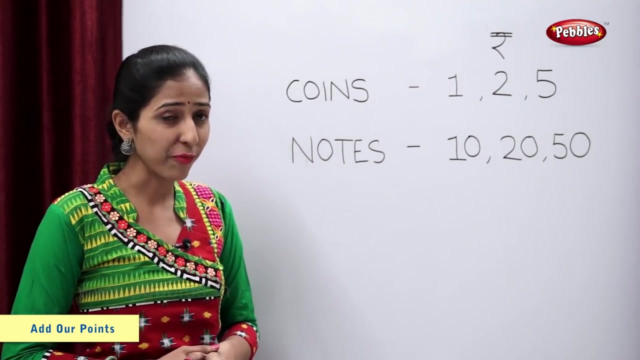 Two at a time, Make a combination of two notes or coins to buy the toys. I wanted to buy some toys, So my mother gave me some coins and notes. She gave me one rupee coin, two rupee coin and five rupee coin. She also gave me ten rupee note, twenty rupee note and fifty rupee note. 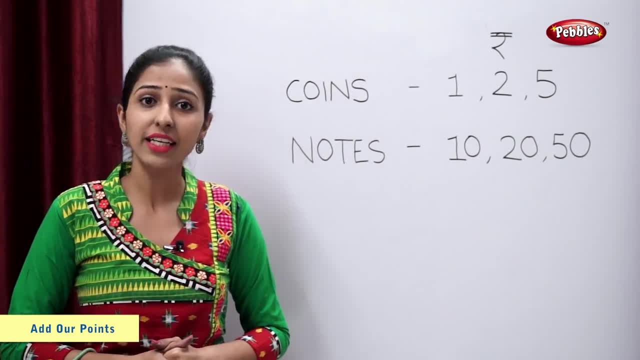 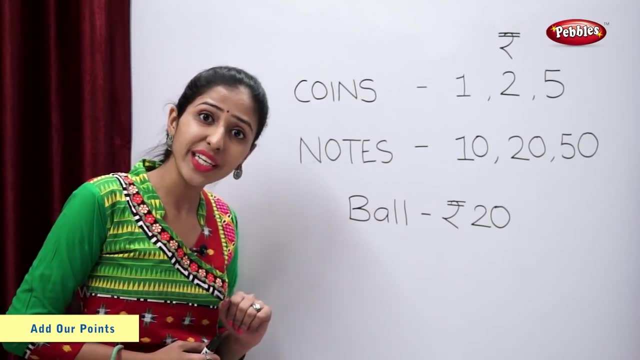 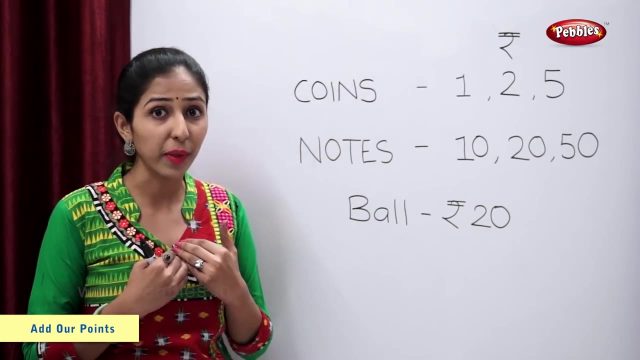 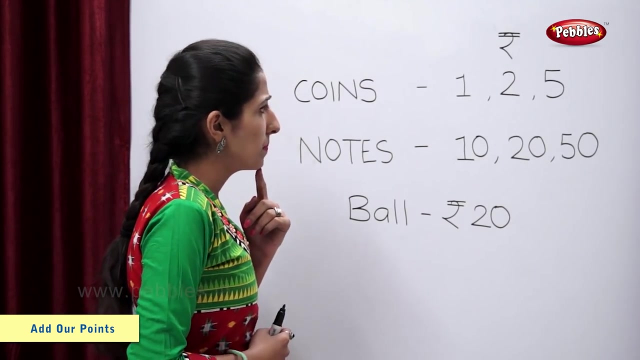 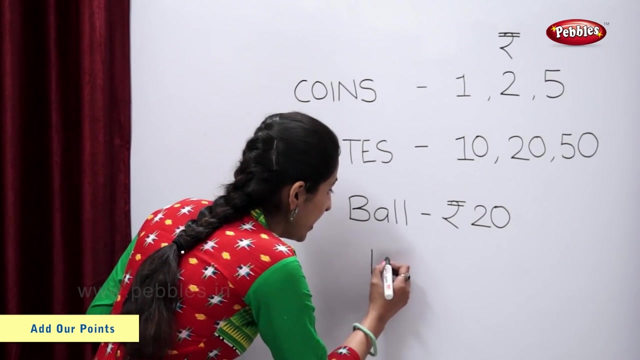 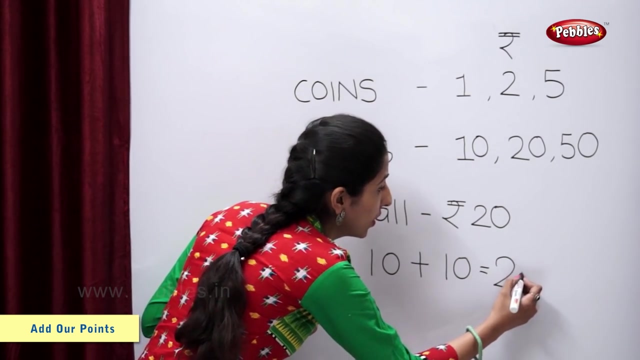 Then I went to the toy shop for buying some toys. I liked a ball. The price of the ball was rupees twenty. So tell me, students, a combination of two notes or coins I required to pay to the shopkeeper To buy this ball. ten plus ten is equal to twenty. So ten plus ten is equal to twenty. 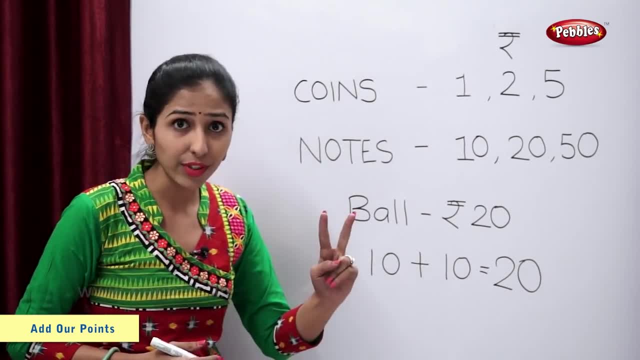 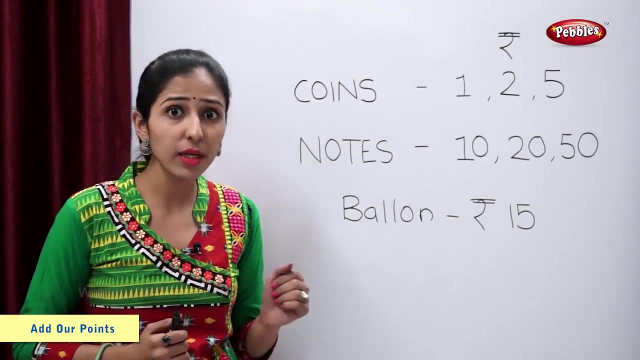 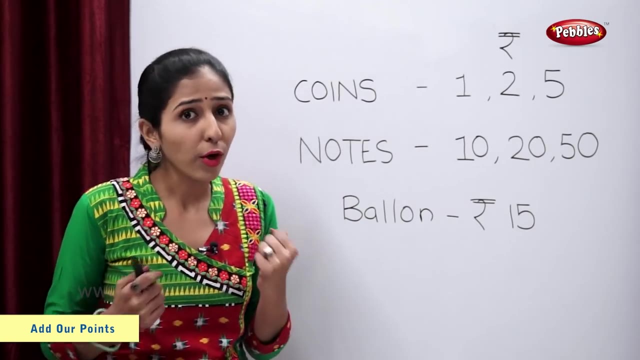 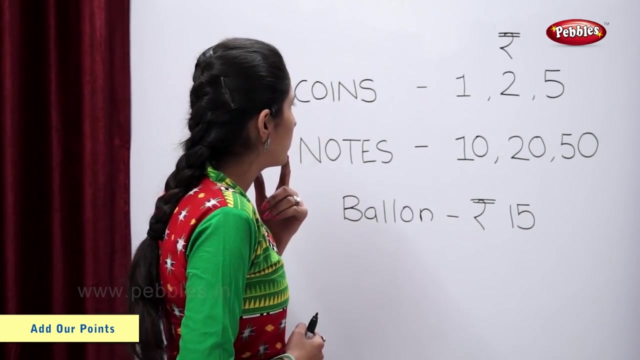 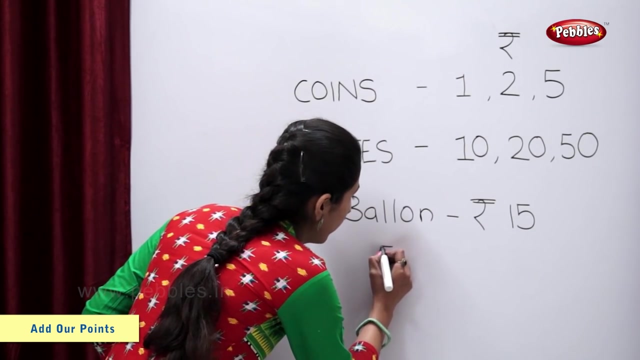 So I will pay two notes of rupees ten to the shopkeeper to buy this ball. I also liked a balloon. The cost of the balloon was rupees fifteen, So tell me what combination is required to make rupees fifteen. Five plus ten makes fifteen, So five plus ten is equal. 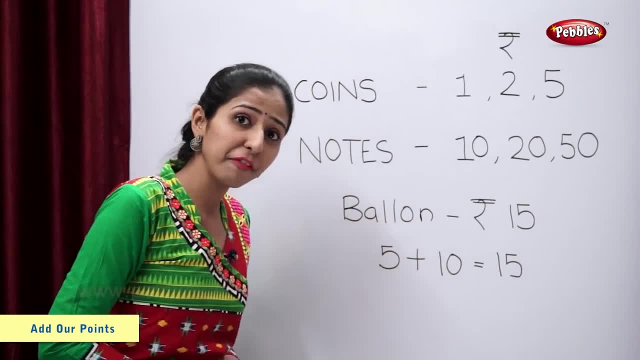 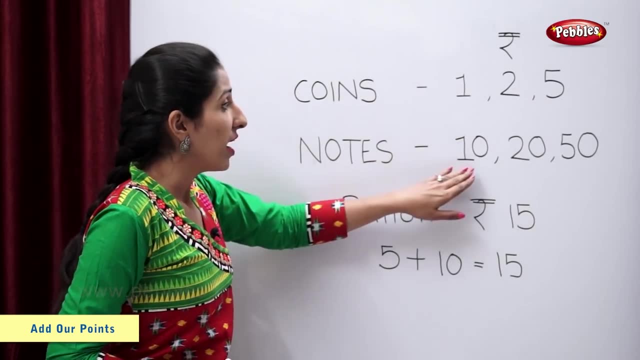 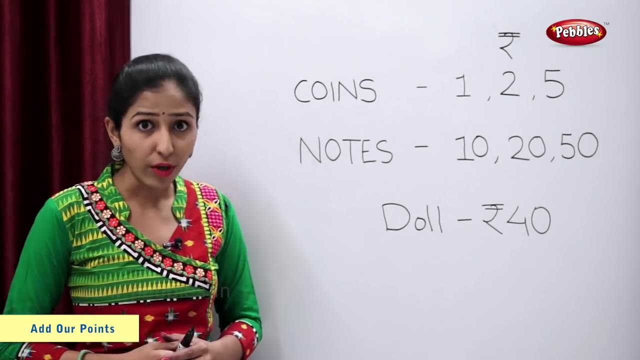 to fifteen. So five plus ten is equal to fifteen. So five plus ten is equal to fifteen Fifteen. So I will pay a five rupee coin and a ten rupee note to buy this balloon. There was a pretty doll. The cost of this doll was rupees forty. So students tell: 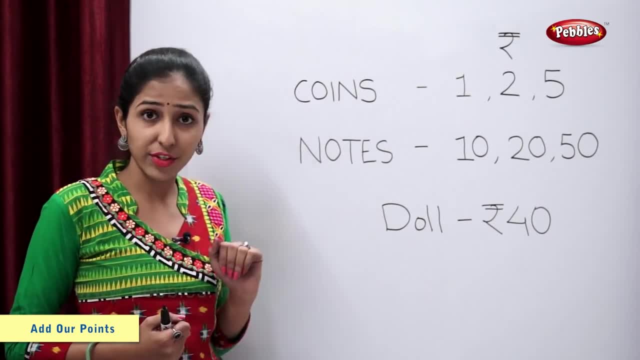 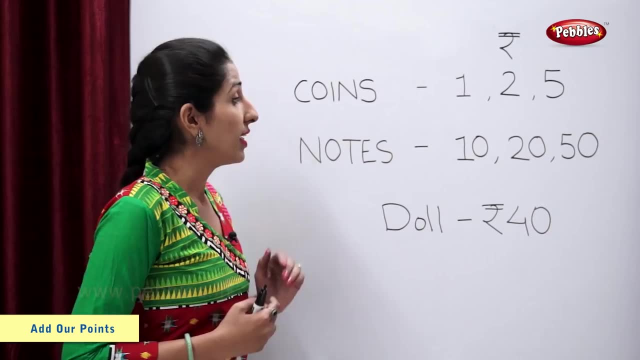 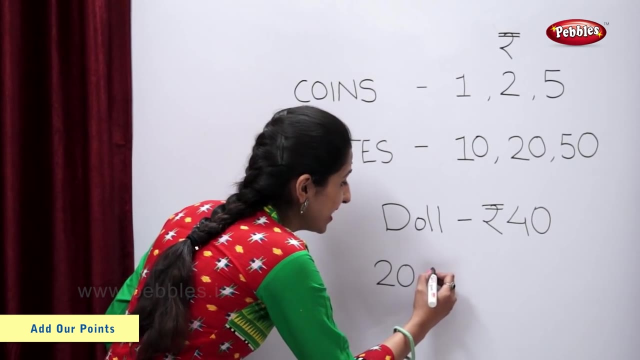 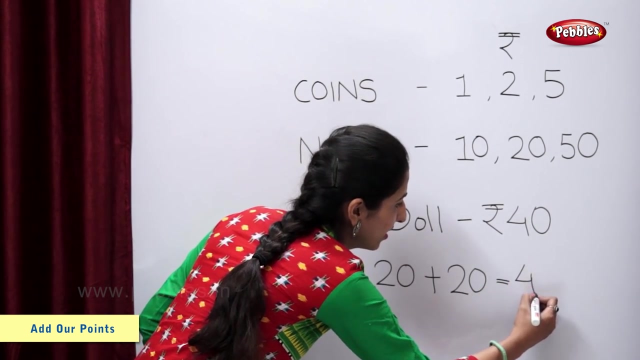 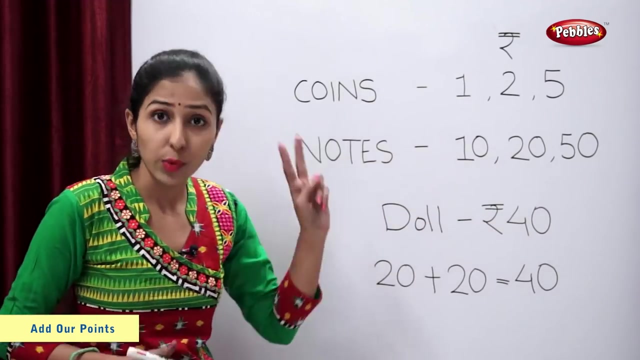 me what combination is required to buy this doll. Twenty plus twenty is equal to forty. So twenty plus twenty is equal to forty. So I need to pay two rupees twenty notes to the shopkeeper for this doll. There was a rupee coin. So students, tell me what combination is required to buy this. 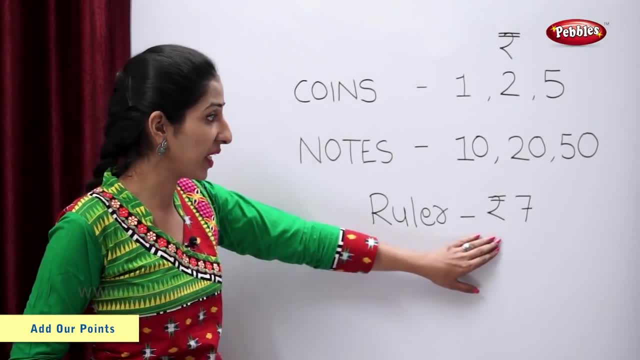 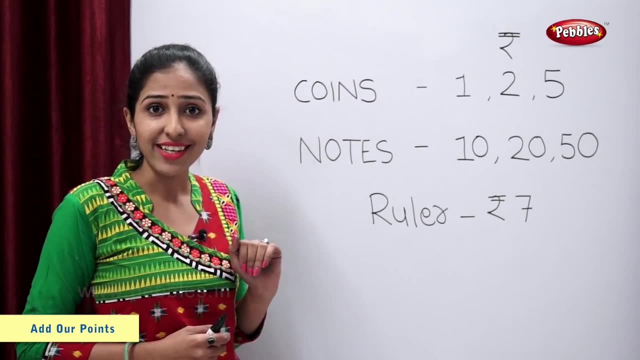 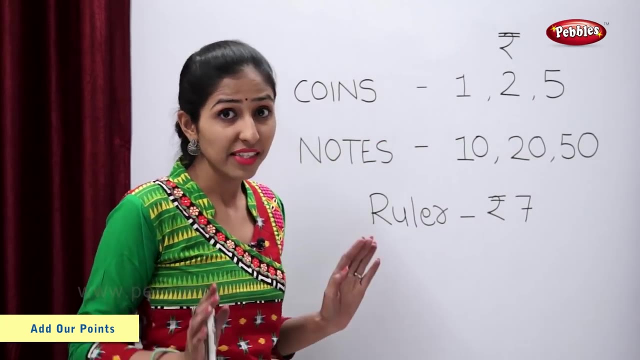 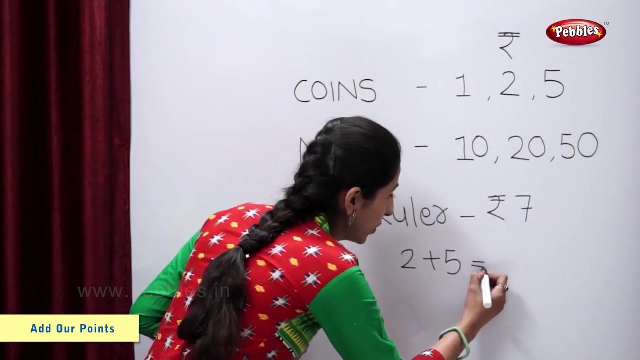 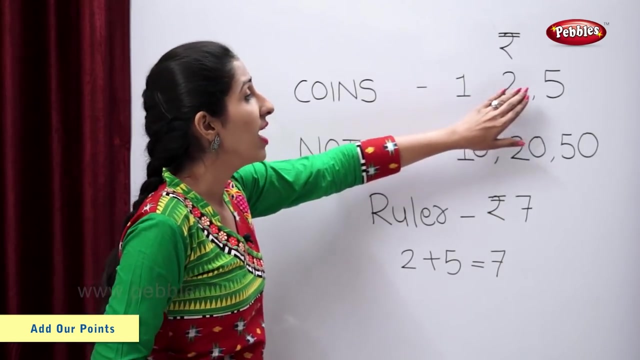 ruler. The cost of the ruler was rupees 7.. So tell me, students, what combination is required to buy this ruler? 2 plus 5 makes 7.. So 2 plus 5 is equal to 7.. So I will pay a 2 rupees coin and a 5 rupees coin to the shopkeeper. There was a book. 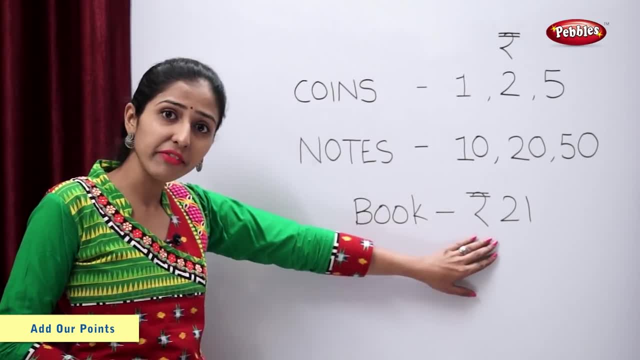 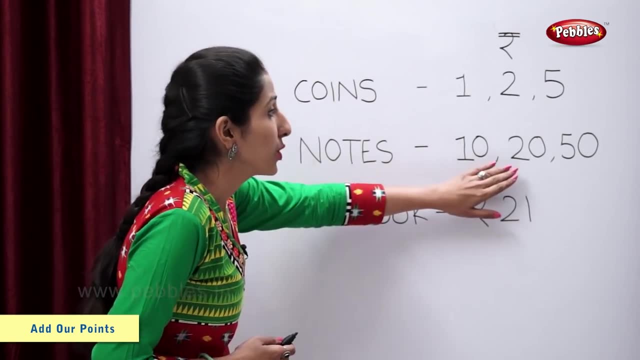 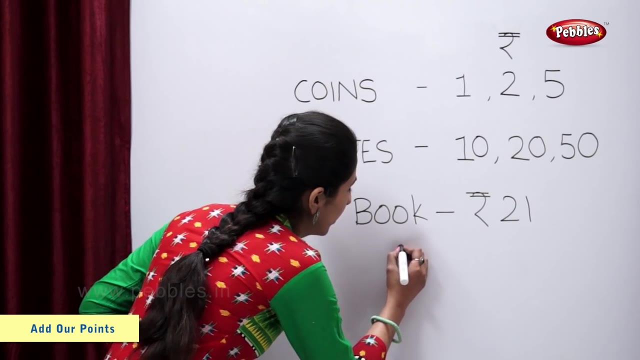 The cost of the book was rupees 21.. So tell me what is the required combination. 20 plus 1 makes 21.. So 20 plus 1 is equal to 7.. So 20 plus 1 is equal to 7.. So 20 plus. 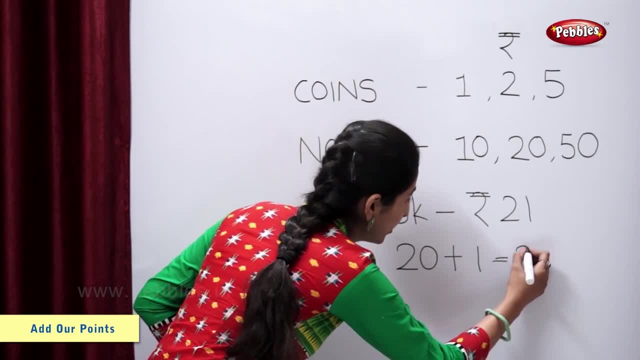 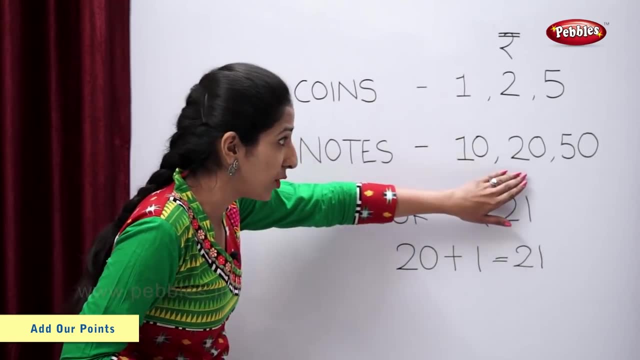 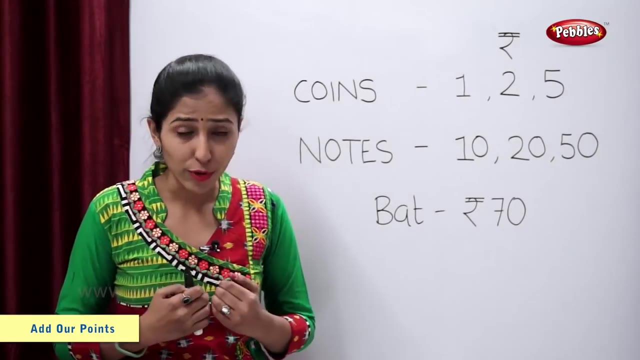 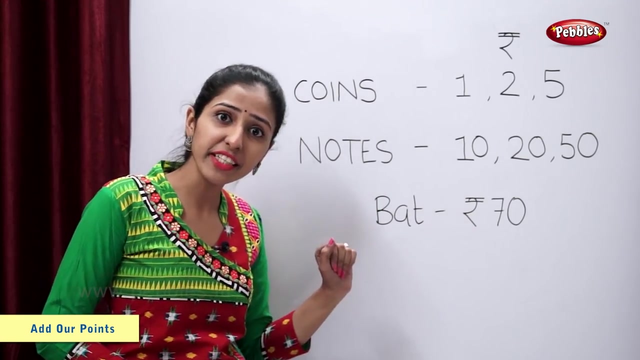 1 plus 1 is equal to 21.. So I will pay a 20 rupees note and a 1 rupee coin to buy this book. I also wanted to buy a bat for my brother. The cost of the bat was rupees 70. So tell. 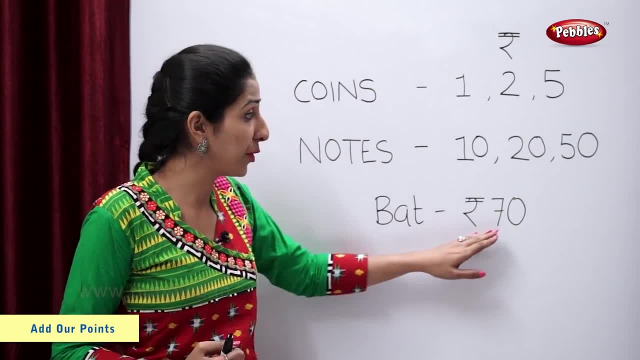 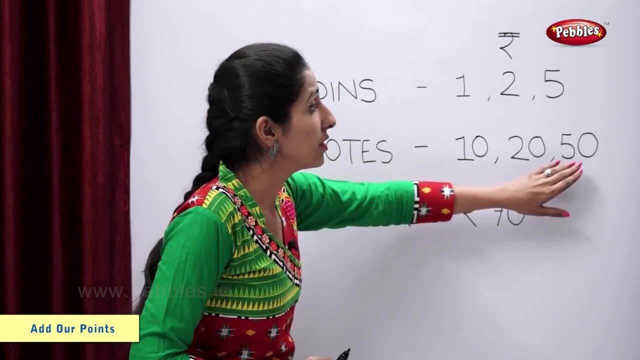 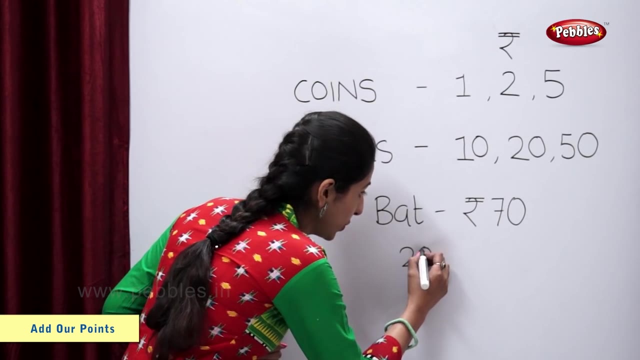 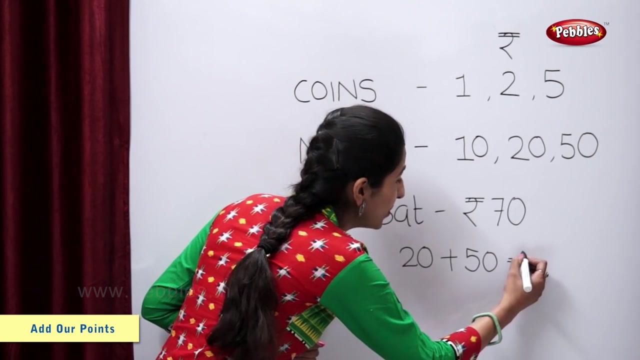 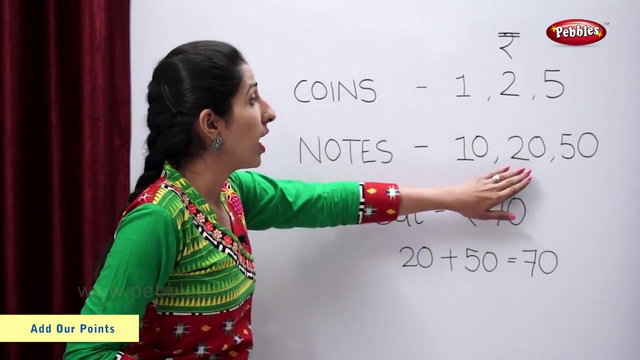 me students, what combination is required to make rupees? 20 plus 50 is equal to 70. So 20 plus 50 is equal to 70. So I will pay a 20 rupees note and a 1 rupee coin to the shopkeeper. There was a book. The cost of the book was rupees. 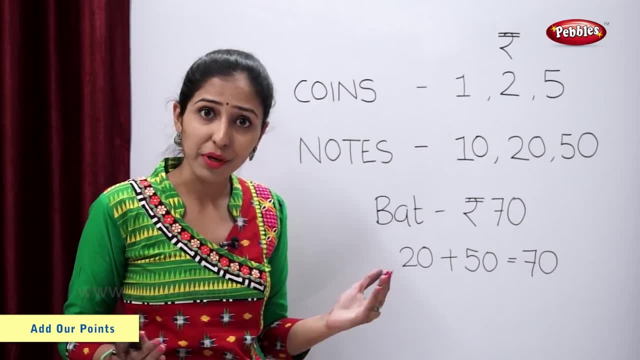 40. So the cost of the book was Rs 15.. So I will pay a 50 rupees note to the shopkeeper to buy this bat.